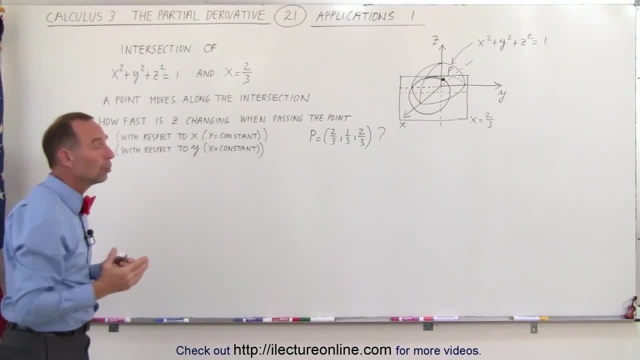 How fast is z changing? Well, what we're going to do- and of course we have to do that with respect to x when y is constant, and with respect to y when x is constant. So let's take the partial derivative of z with respect to x. Now, if we're going to do that, we have to rewrite the equation. 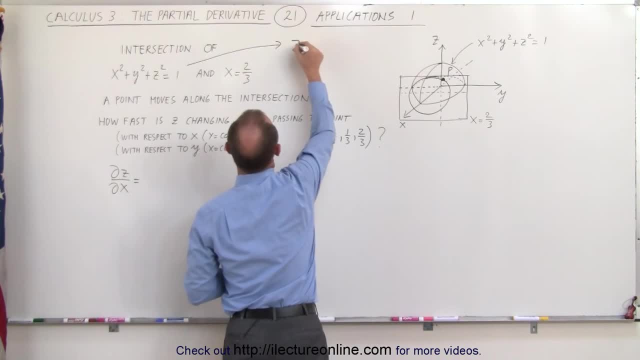 We have to write the equation as follows: z is going to be a function of x and y, which means that z is equal to the square root of 1 minus x squared, minus y squared. So now we take the derivative of that with respect to x, which is equal to 1.. 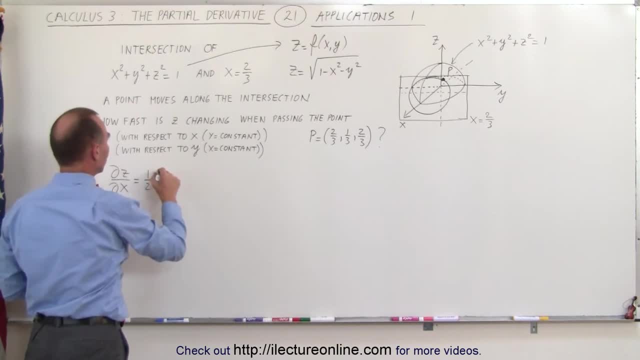 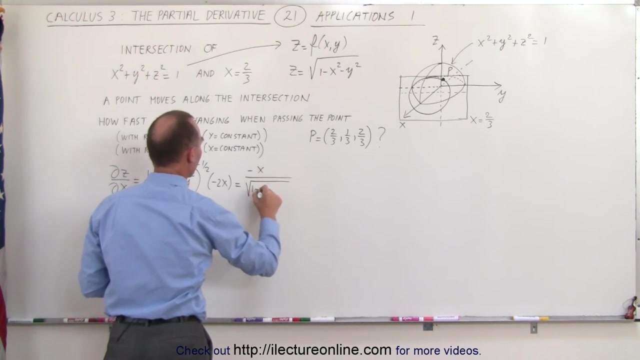 One-half times the 1 minus x squared, minus y squared, to the one-half minus 1, which is minus one-half times the partial derivative what's inside with respect to x, which would mean minus 2x, and this, therefore, is equal to minus x divided by the square root of 1 minus x squared. 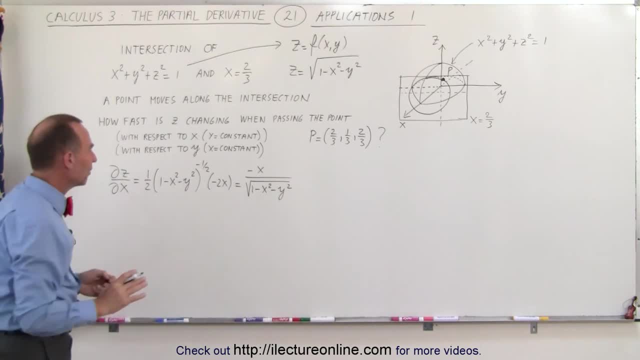 minus y squared. Now we're going to take the partial derivative of that function with respect to y. The partial of z with respect to y is equal to one-half times 1 minus x squared, minus y squared to the minus one-half times the partial derivative. what's inside with? 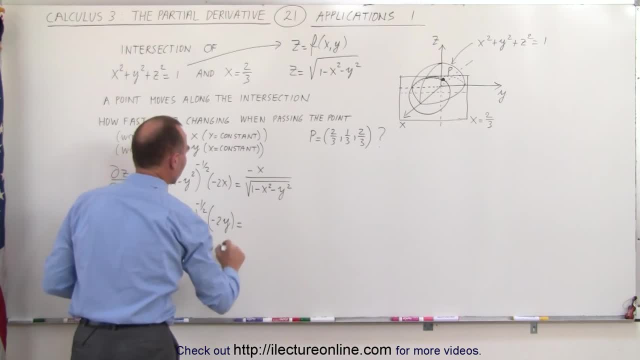 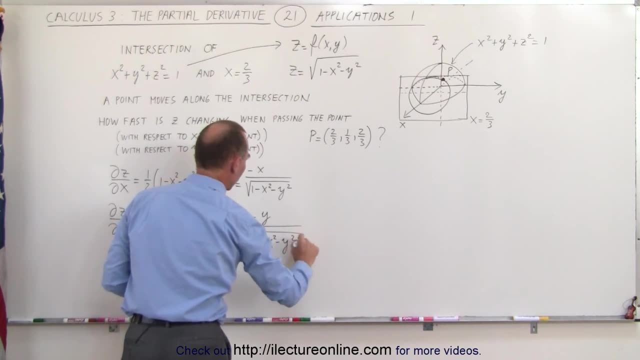 respect to y, which is minus 2y, and therefore this becomes: minus y divided by the square root of 1 minus x squared minus y squared. What we need to do next is we need to plot the derivative of z with respect to y, which is minus 2y, and therefore this becomes: 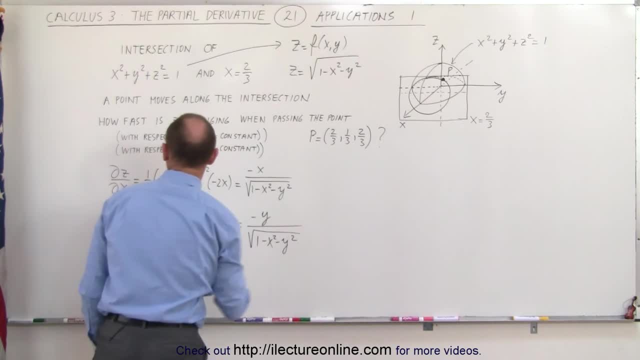 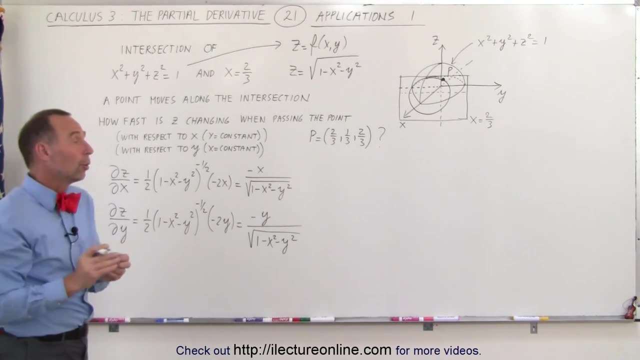 minus 1.. So we're going to plug in the values. So now we can evaluate the change in z with respect to x and the change in z with respect to y When we plug in these values, because we want to know what the change in z is when we're at that. 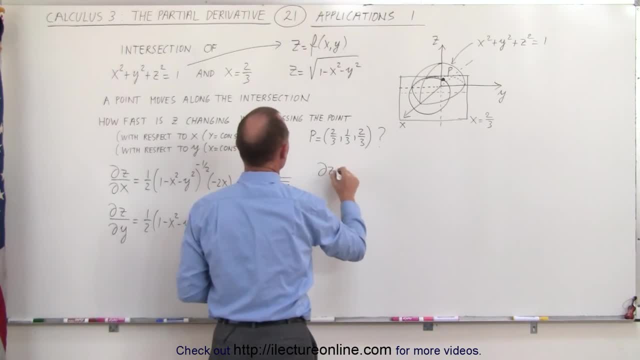 particular location. So the partial of z with respect to x is equal to, and of course we're going to plug in the values for x and y- two-thirds for x, one-third for y- and this is going to be equal to 1.. 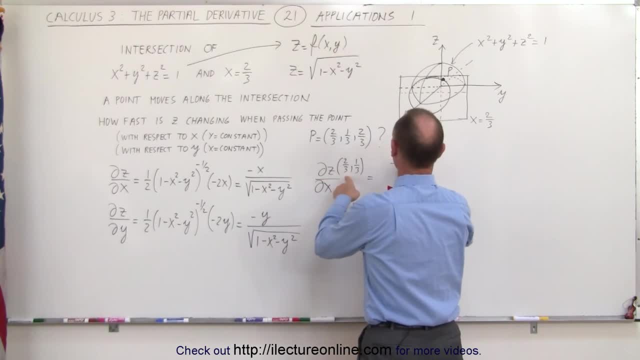 minus x. now x is going to be 2 thirds. so it's minus 2 thirds divided by the square root of 1 minus x squared, which is 2 thirds squared, that would be 4 ninths minus y squared. 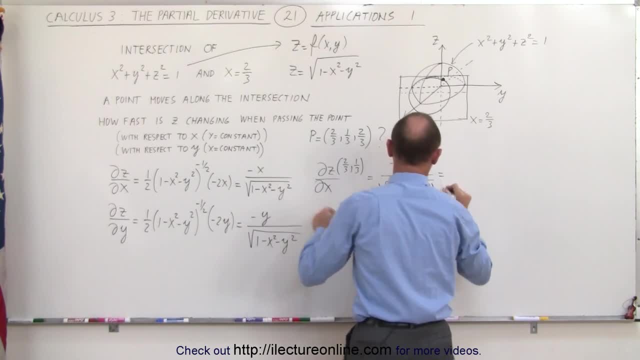 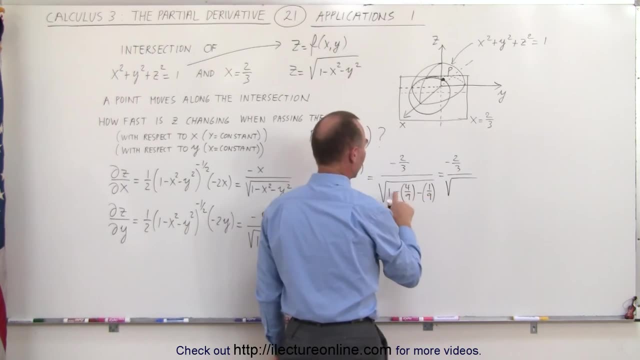 which is 1 third, squared which is 1 ninth. So this becomes equal to minus 2 thirds divided by the square root of that's 1 minus 5 ninths, which is 4 ninths, which is equal to minus. 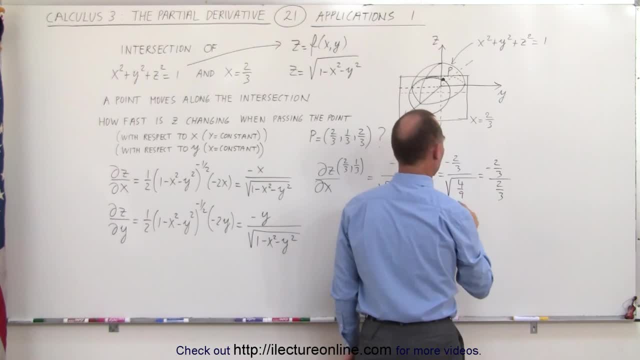 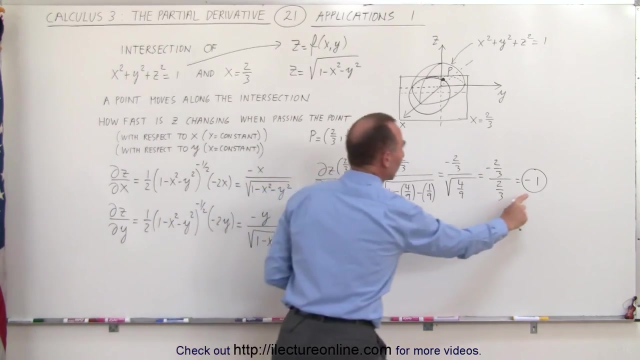 2 thirds divided by 2 thirds and minus 2 thirds divided by 2 thirds is equal to minus 1.. So that means that the rate of change of z with respect to the variable x- when y is constant, it is equal to a negative 1.. If I now take the partial of z with respect to 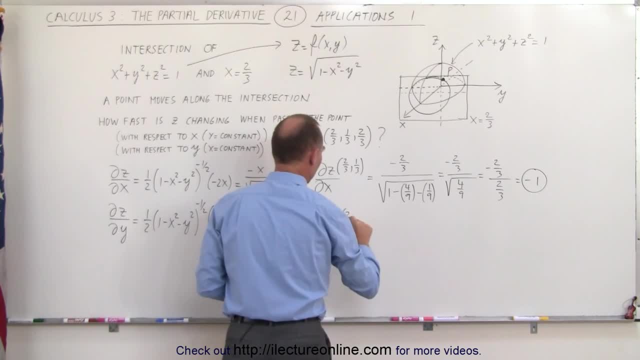 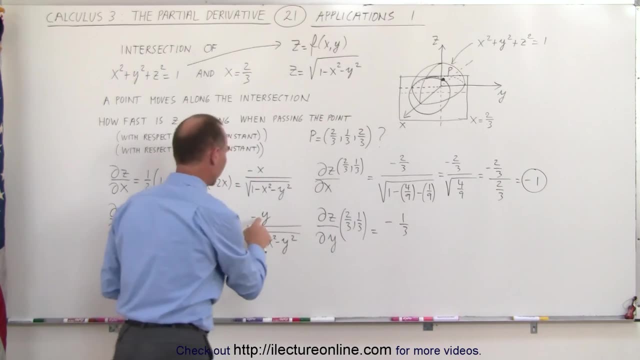 y and I plug in the values for x and y. this is 2 thirds and 1 third for x and y. that is going to be equal to minus 1 third, because I'm plugging in 1 third here for y divided by the square. 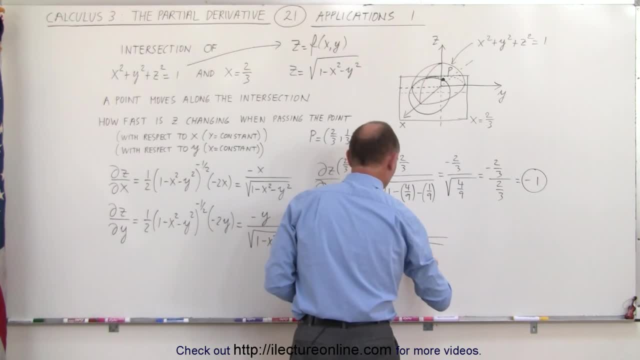 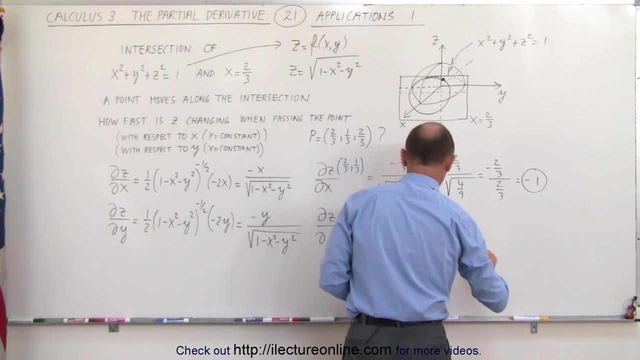 root of the denominator is going to look exactly the same. that would be 4 ninths and minus 1 ninth, which means this is equal to minus 1 third divided by the square root of 4 over 9, which is equal to minus 1 third divided by 2 thirds, which is equal to minus. 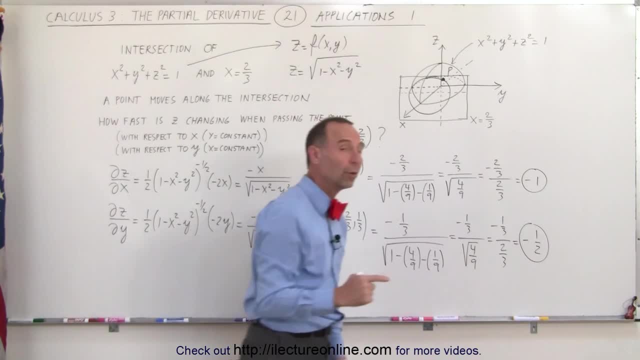 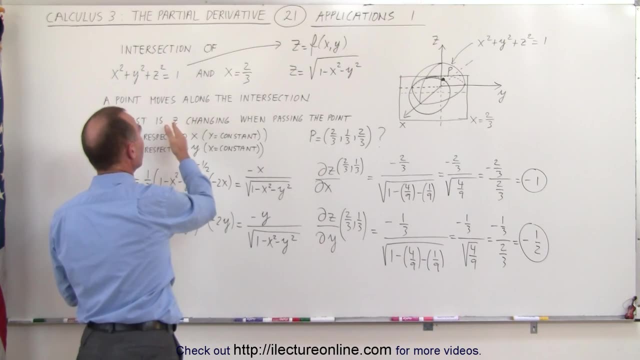 1 half. So that's the rate of change of z With respect to y, as x remains constant. and so that's what we're doing here: we're trying to find how fast z is changing when passing that particular point with respect.